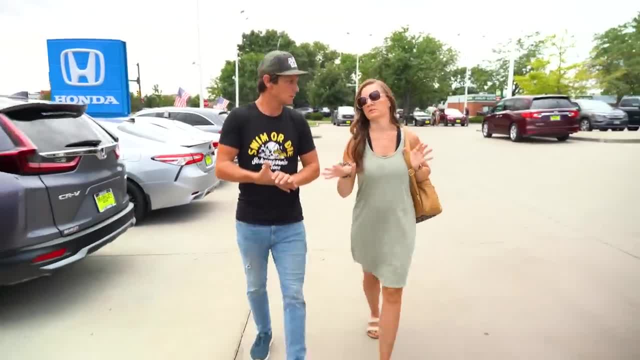 Okay, let's just go look at a minivan, but not for serious, For sure, Not seriously Like a joke. Yes, it's just a joke, So that we know that, we know that it's stupid. Exactly, We can just put it to rest. 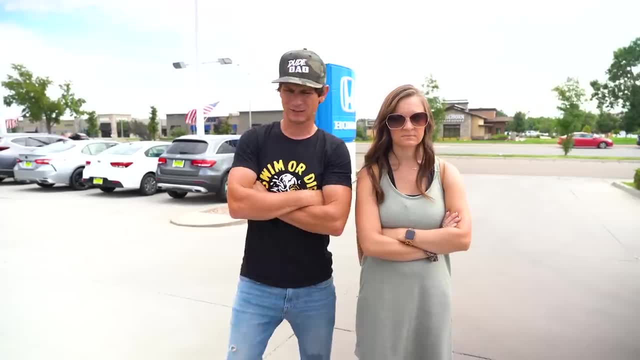 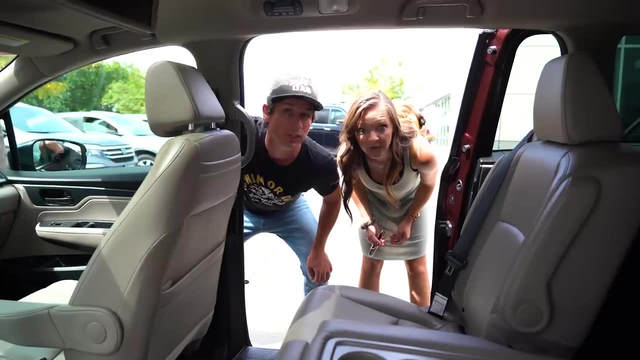 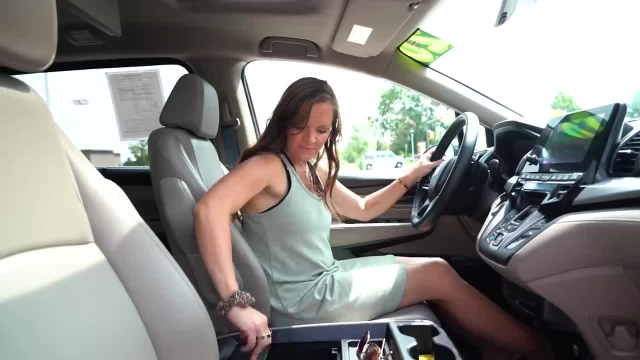 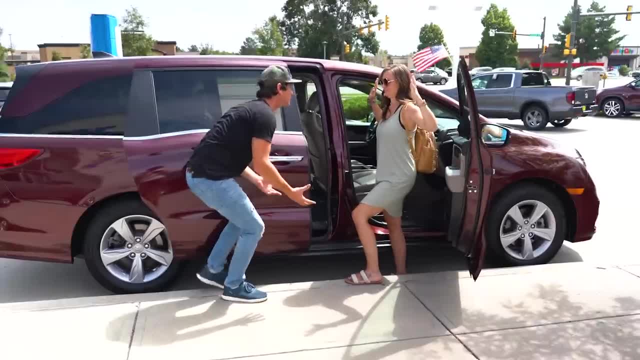 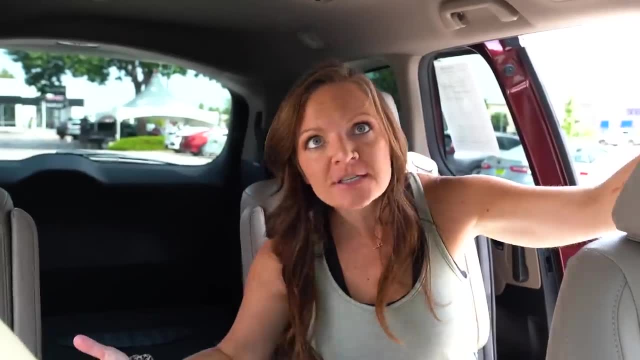 What Babe? there's trash bag, hooks, What? No hands. It's a freaking spaceship. Oh, that is a game changer, A Blu-ray player. Why is there a Blu-ray player? Because there's a TV. It's got to be like nine inches. 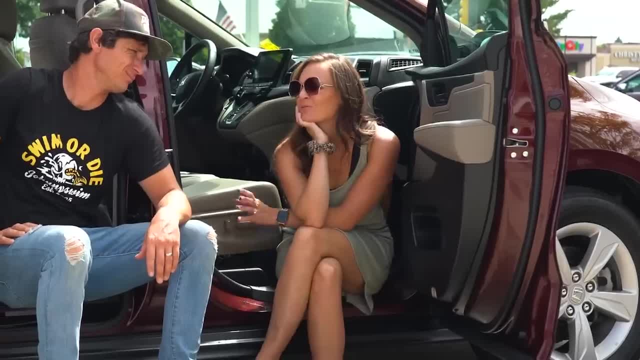 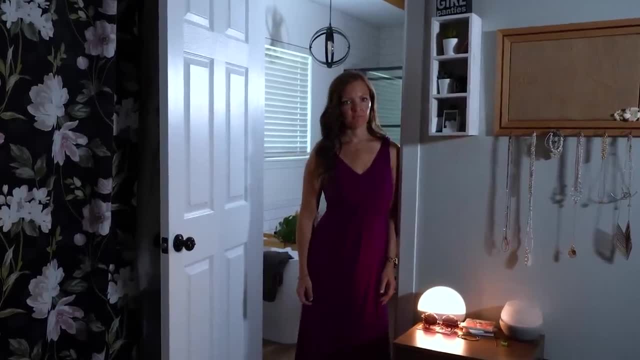 Nine inches, Yeah, but it's still a minivan. We would never. We would never, Ugh, Ugh. I need to say something, but I'm scared to say it. It's okay, I know what you're going to say. 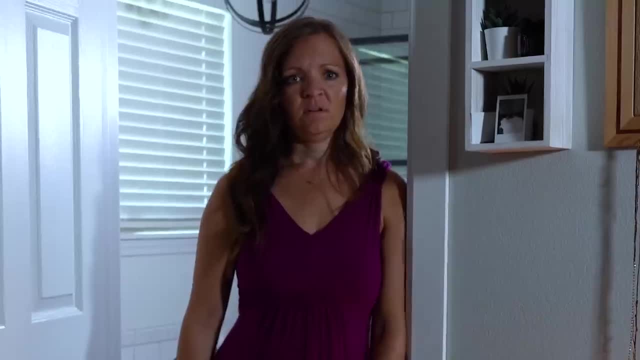 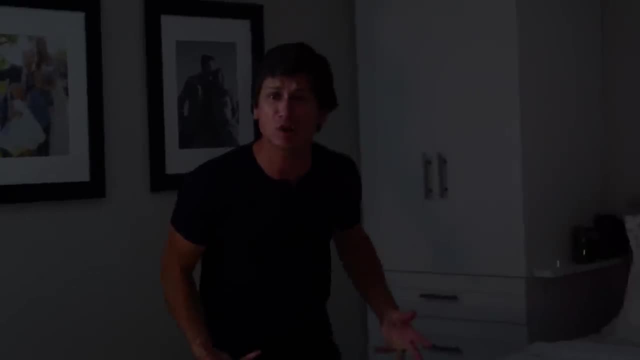 You think we should get a minivan? Ugh, It sounds even worse when you say it. I know We're not minivan people, but we can't deny how ridiculously functional they are. Taylor, be honest, Will you find me less attractive if I drive your minivan? 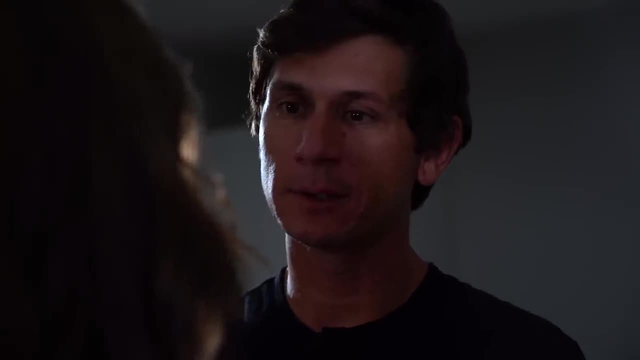 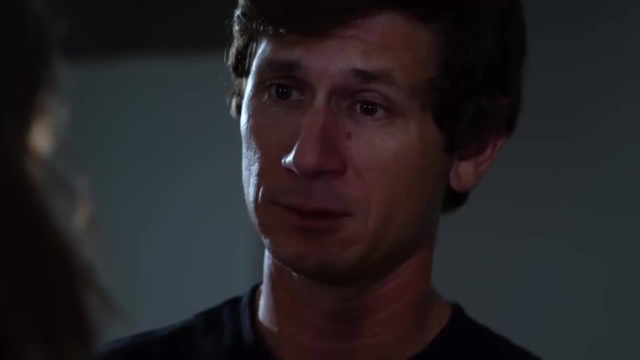 Of course I will. I understand, But at the same time I will find you ridiculously attractive for having the courage to drive around in a trash can on wheels. Promise me, we'll tint the windows. I promise What I know. Isn't she sexy? 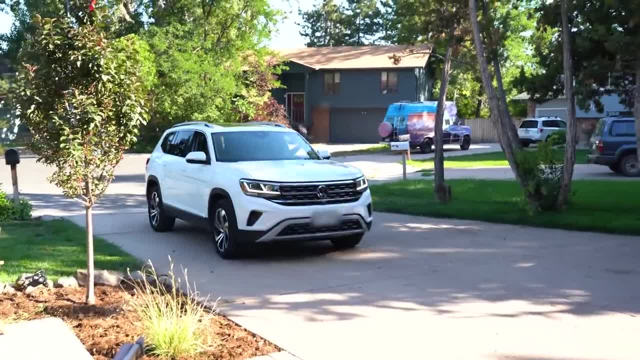 For sure it is, But what happened to the minivan? We don't need it. This thing has a third row and some of the features of a minivan. Ha, Some features, That's enough. I wish I was confident enough to drive a minivan, but I'm just not there. 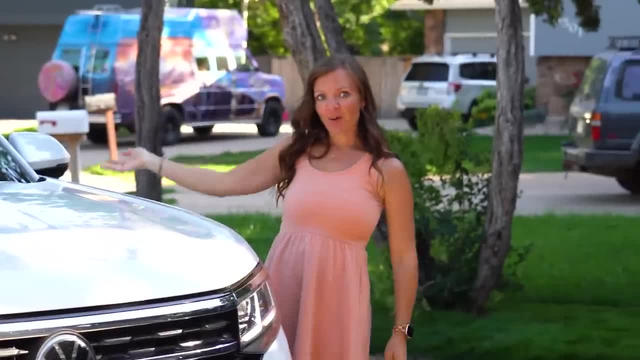